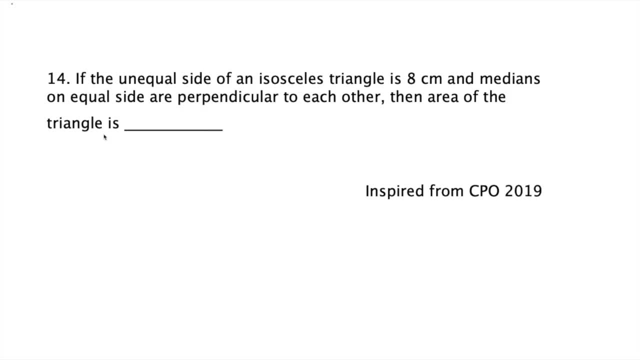 Hello friends, welcome again to the world of maths by MEA. So this one is one of the easiest question I am going to solve in the must before examination series. I know this is quite easy question. If you have solved it before, I would suggest please post the answer in the comment box. 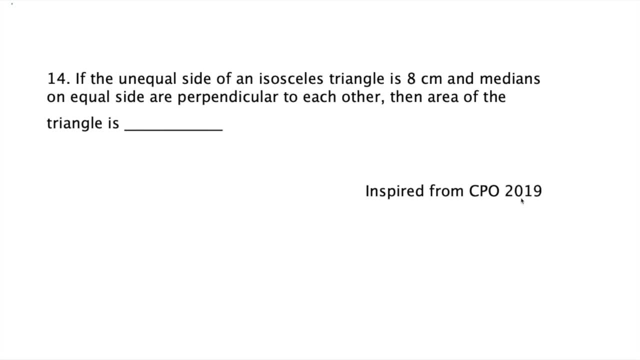 because I have said this question in the Facebook group too, and this question is inspired from CPO 2019 paper. I would suggest please pause the video and try to solve this question if you have not solved it yet. So I hope you have paused, solved and answered the post. This is quite easy. So at 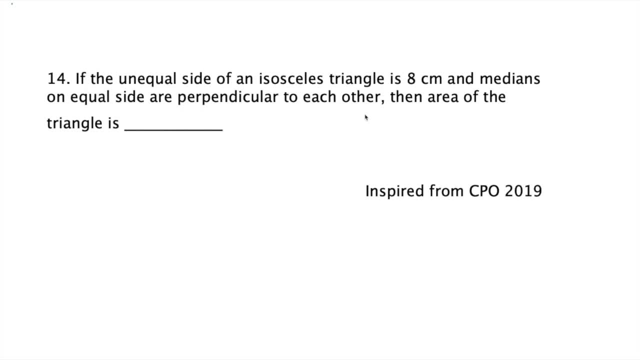 a first glance this seems to be a question of medians. perpendicular means a square plus b square is equal to 5c. square is the formula if the medians are perpendicular. But we can solve this question with the basic logical concept. Say this one is an isosceles triangle in which 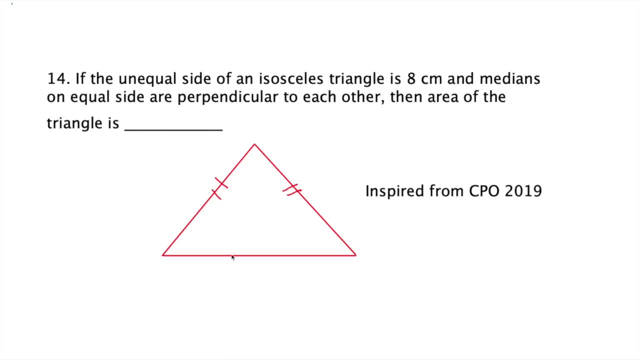 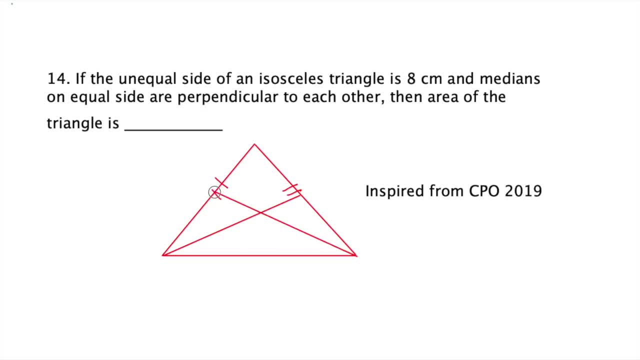 the equal sides. So these are the medians on the equal sides. Fine, And assume these medians are the perpendicular- It's not visible, as per the figure, but assume this one is a perpendicular means 90 degree at each sides. So I'm going to use a simple concept of the median, If you have. 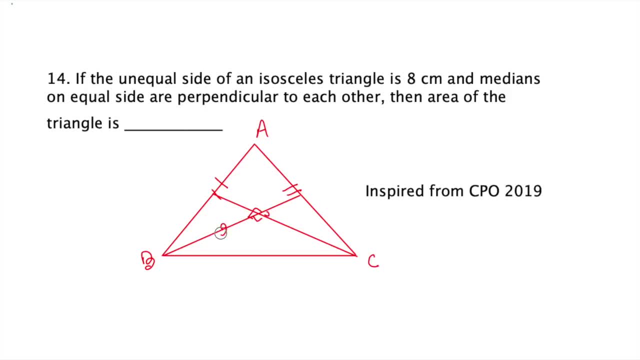 isosceles triangle, then the median should equal. So if I say this one is 2x and x, why I have taken the 2x and x? because I know median divides in the ratio of 2x and x, So this is also the 2x and x. 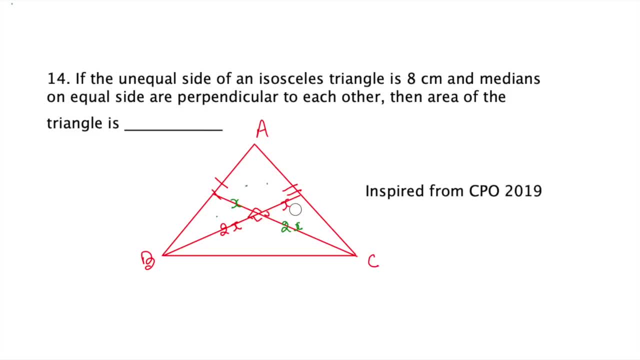 And we know medians divides triangles in six equal parts. So if I can find the area of this one which was nothing but half into 2x and 2x, how comes 2x and 2x half into base, into height? 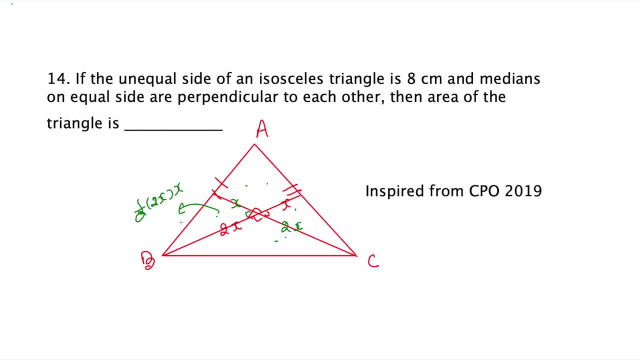 because this one is 90 degree. Assume this one is 90 degree. Figure is not as per scale. So if I am able to get the value of x squared and I multiply it by 6, I get the value of complete triangle. How comes First of all, if I can find the area of this small triangle? I know the area of. 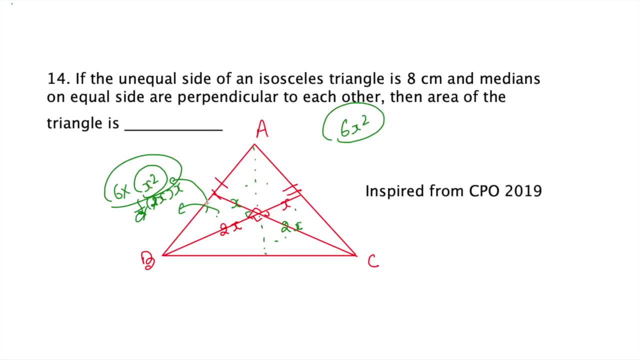 all would be divided into six equal parts. If I can able to find the value of this triangle, that is, half into 2x into x, if this one is a 90 degree, If this one is a 60 degree, then half into.